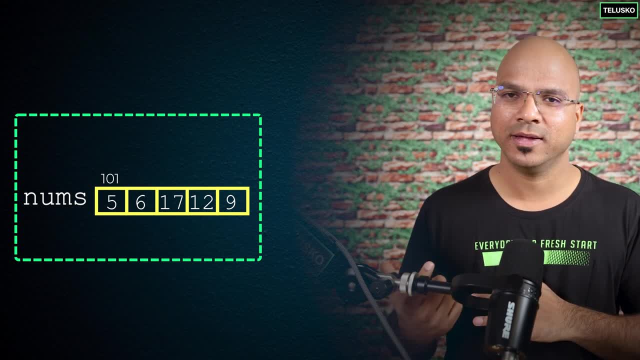 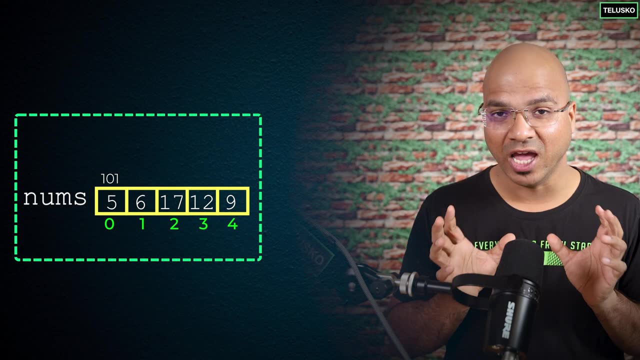 the first element is: look, is at 101. So it will have an index value which is zero. the second element is one, then two, then three, then four, right Now for five values. the index value starts from zero and ends at one. So if you take a value of a value, you will get a value of a value of a. 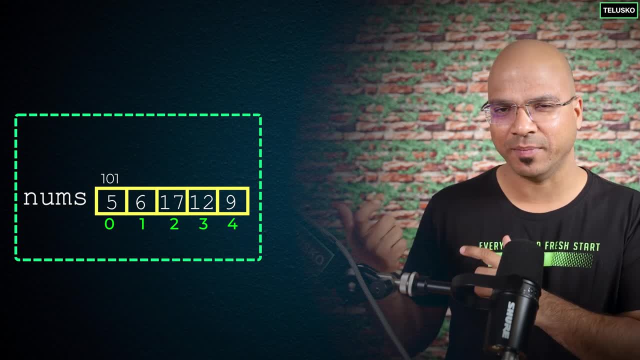 value. So that's why we have to use an index value. So let's say the first element is at four. Now, why zero? is because we start. we have a memory allocated right, One zero one which represents the first element, so we don't have to give one to it. So what you do is the next element is plus. 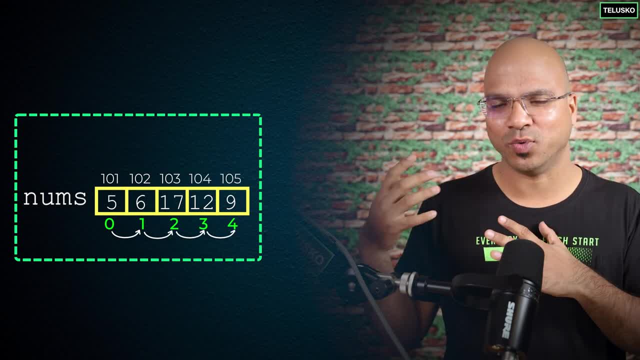 one. that's why 123.. And then you can just get it right. So one zero one. let's say, if you want to get the third element, you have to say plus two. that's how you do it. So you got the values. 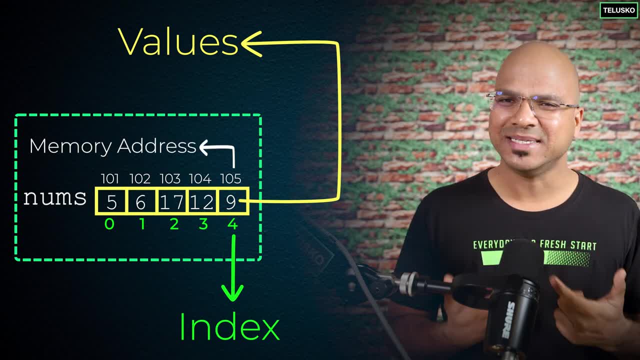 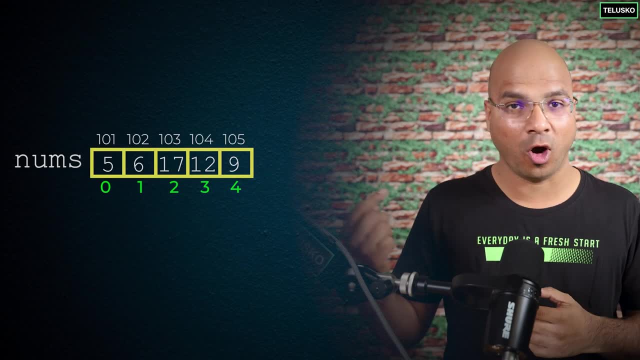 you got the index and you also got a memory address to it. Now, with this array- as we already talked about ADT, which is abstract data type, we should be able to perform some operations. Now, what option you can perform on this array? now we can perform something called a read operation. So 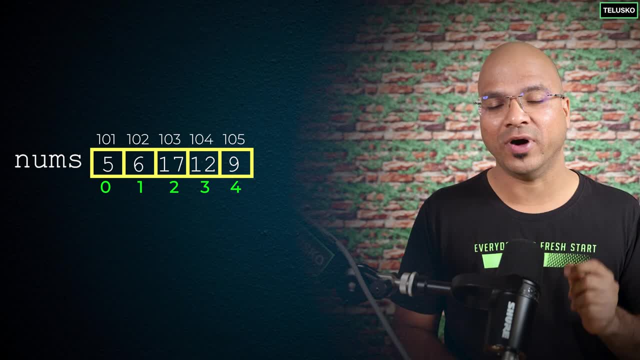 what is read. So let's say you want to get the value of index number three. Now what? what you do in this case is you say, okay, my array name is nums And then for this nums, I want the value at index three. So in different languages we have different representation for this. But let's say 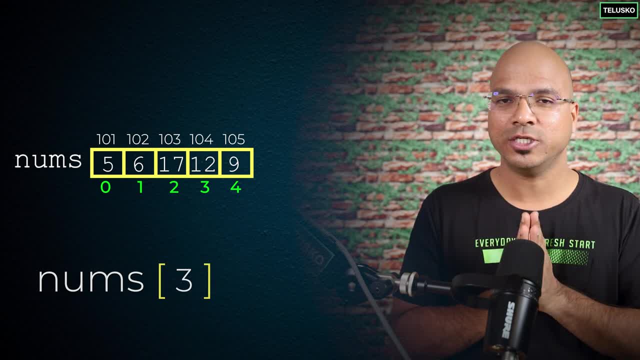 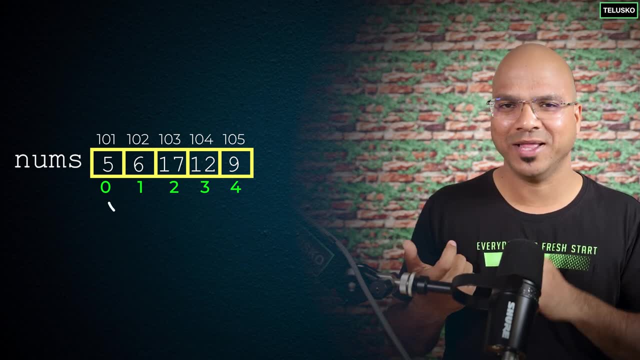 this is common one, So nums bracket of three. Now what your computer will do is it will directly jump to the memory address. It's very simple for the for that right. So you will say one zero, one plus three. you will get the value. So that's how you do it. Now reading is very easy And 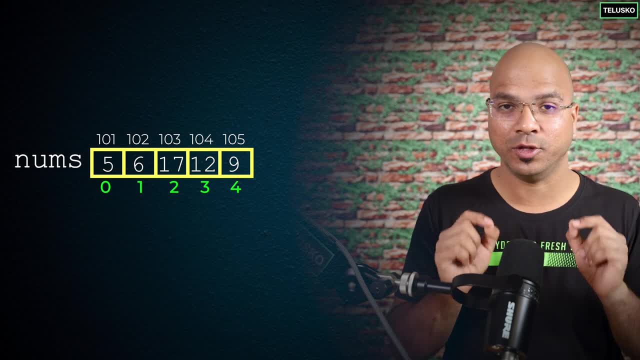 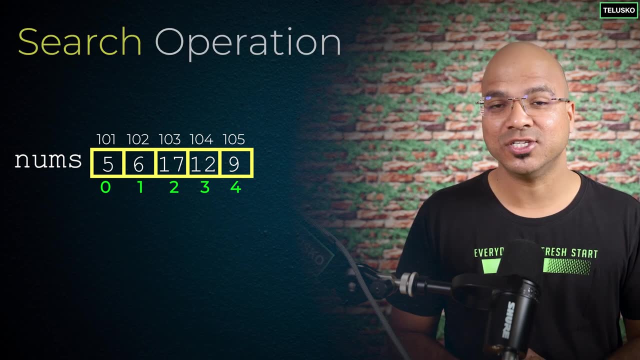 computer takes way less time to jump to that particular area is because the computer knows the memory right. Because you are mentioning the index value. Reading is good, It's fast. also, What about searching? Now, this is tricky, because when you're searching, you're not searching for. 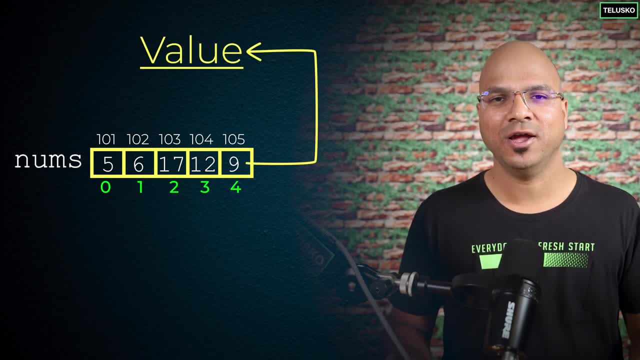 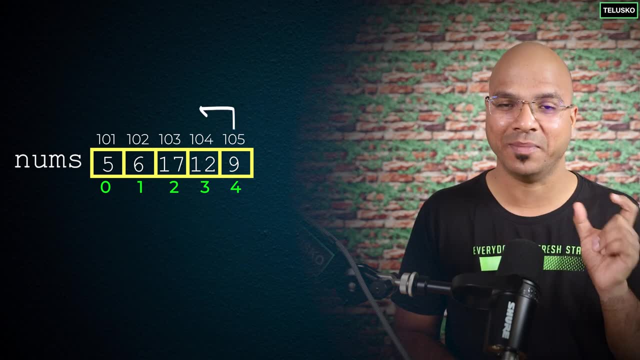 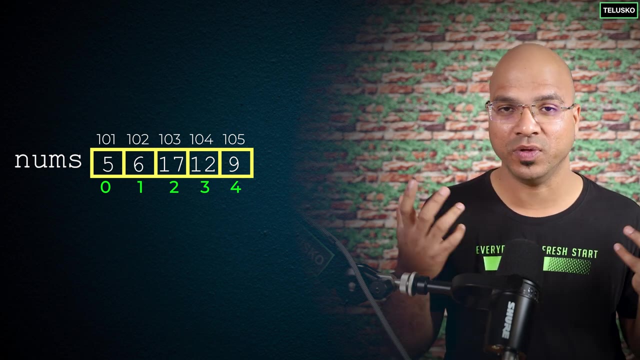 an index. you are basically searching for the value now. So let's say, from this array I want to search where is 17.. Now, in this case, your computer has no idea where 17 is, because computer has no idea in which location we have that value And do we even have that value? So what a computer. 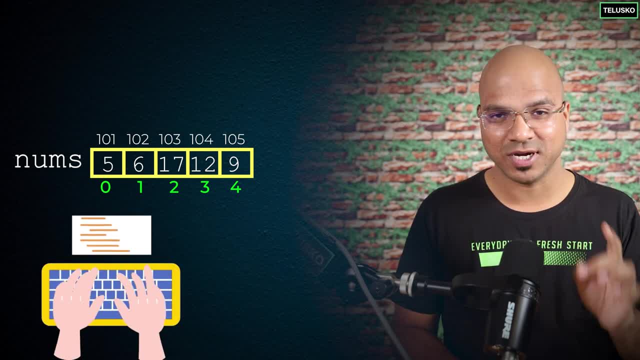 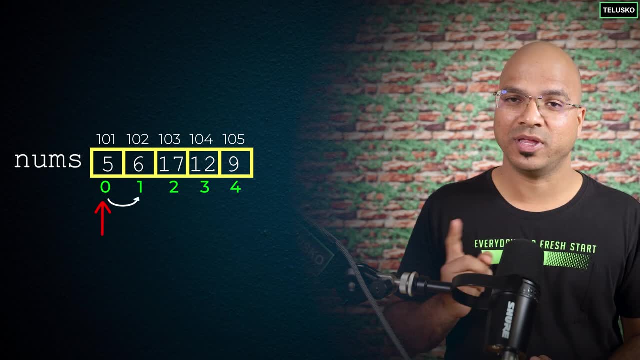 will do is it will start on the first location. So basically, you have to add a code to search from the first location. you have to check. is the first one 17?? If yes, good, we can exit. No, then you have to jump to the next location. Is it matching? If yes, good. If not, next Matching: Yes. 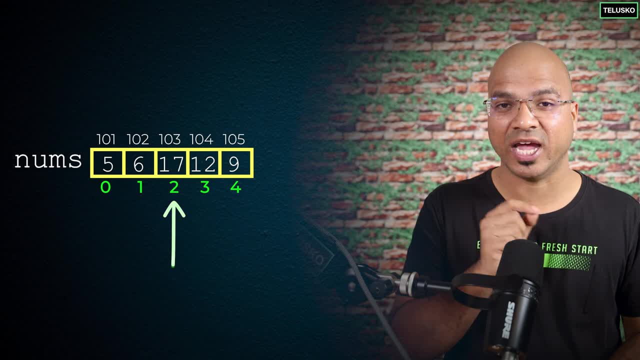 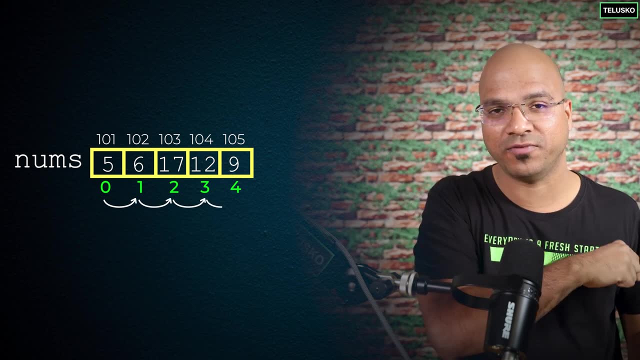 no next. So basically, you have to search each element, right? And let's say the element is at the end. you are searching, you are basically tracking to all the different locations. So this is time consuming, right? What if you have a array of, let's say, 1000 values to? 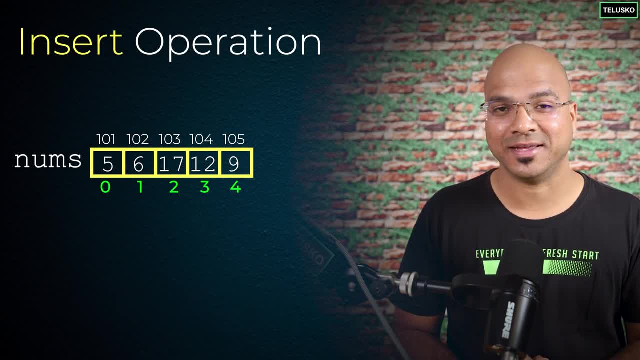 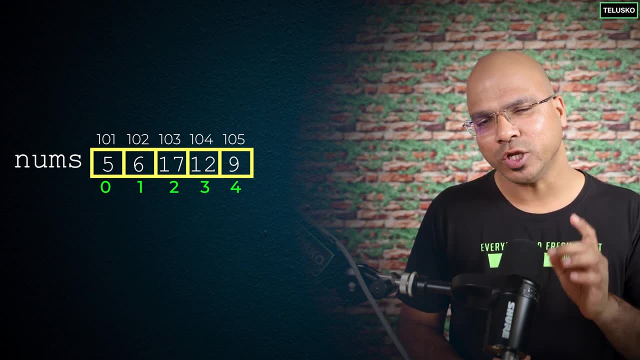 move between these values. it will take some time. What about inserting? Now, this will be tricky is because, see if you want to insert an element, what do you think Will it? will it take a lot of time? See if you want to insert the element at the end? that's very simple. you can get the 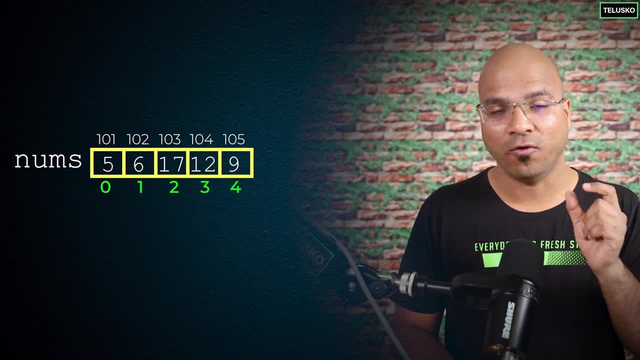 size of the array, because we also have to have that option of getting the size of the array. let's say you have five values. you will simply jump to the sixth location, which is index five, And then you will say: okay, I want to add a value here. let's say the value value is 21.. And you can. 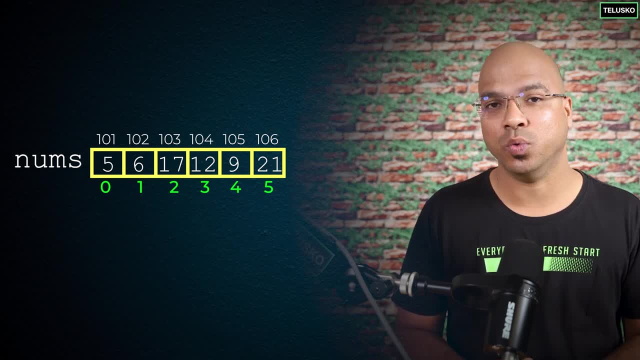 add the value. it's very fast. But what if you want to add a value in between? So let's say you want to add that value at the second location, So after the first, you want to add the new value. Now what you will do is you don't have a space there, right? you can't simply create a new space. you can create. 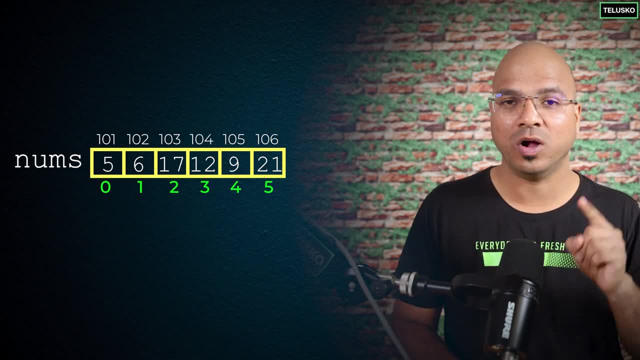 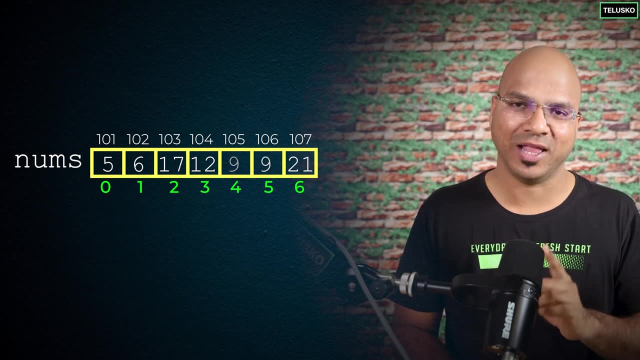 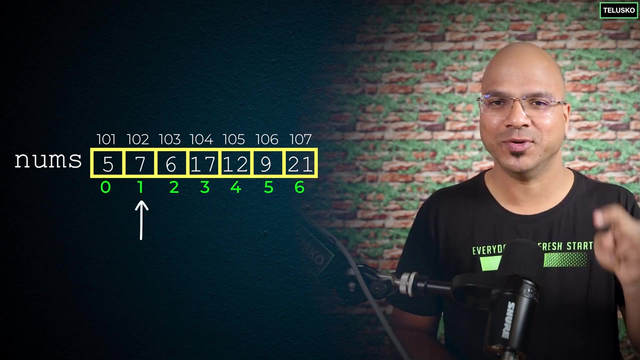 space at the end. So what you do is you basically have to move all the elements, And it's not like move the elements, what you do is create a new block, So move the second, last element now to the last block. then again, you have to move every element one by one. then you can add your value. 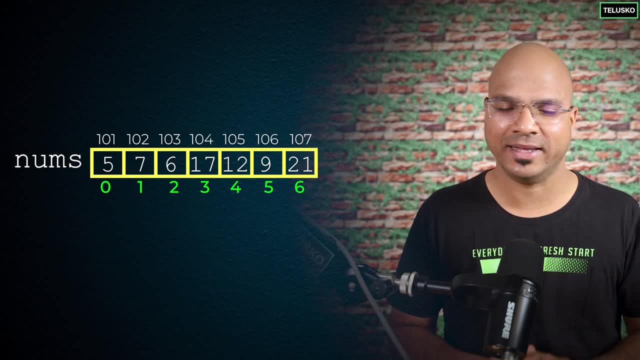 to the second location. So if you are inserting at the end, that's fine, But if you're inserting in between, that will take a lot of time And that depends upon the number of elements after the position which which you're adding. What about deleting See? deleting from me from the end is. always welcome is because you're not affecting your argument, So you can add that value at the end. So if you're working in the beginning, you can add that value. but if you're working in the beginning, you can add that value at the end. So if you're working in the beginning, you can add that value. 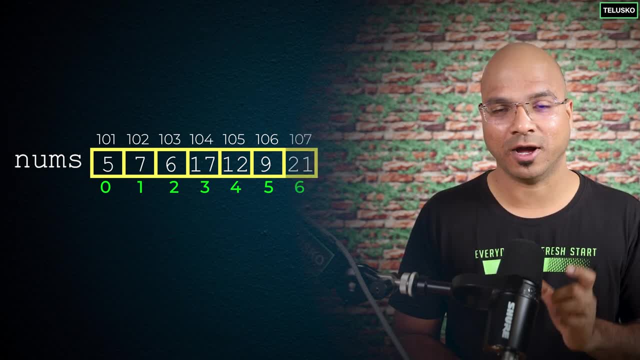 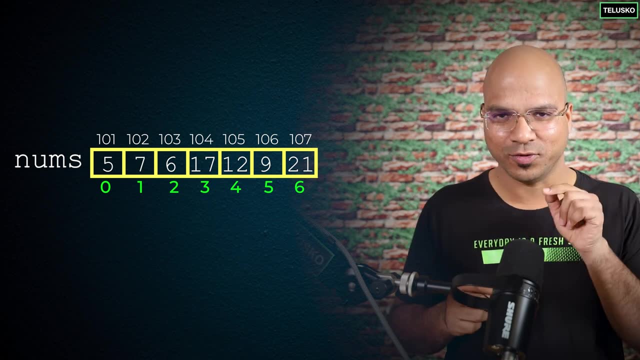 array in total. but what if you want to delete a particular element from between? now, you can't simply delete from the between right, you have to delete the end block. but how will you move? so again when you, when you want to delete this, just replace all the values, right, so that's, that's. 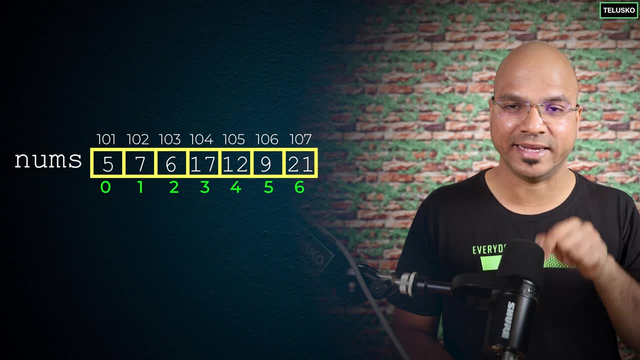 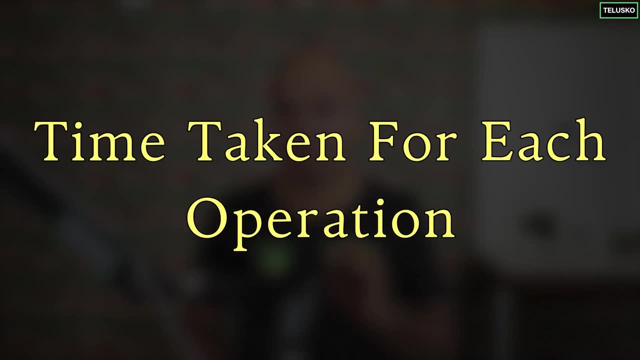 tricky, so it will take a lot of time, depend upon how many elements you have after that index value. now, while we are talking about all this thing, array was simple, right, we can perform the operations. the important thing here is time taken for each operation, and it's not about cpu time, if you're. 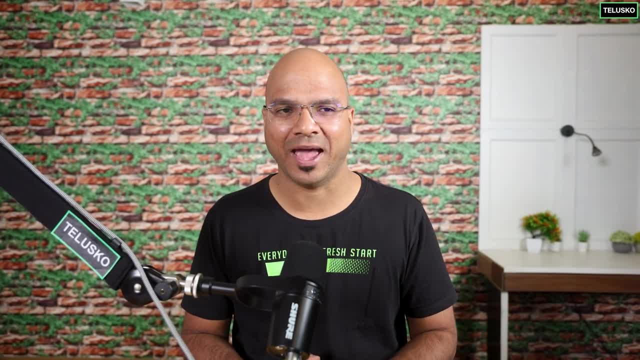 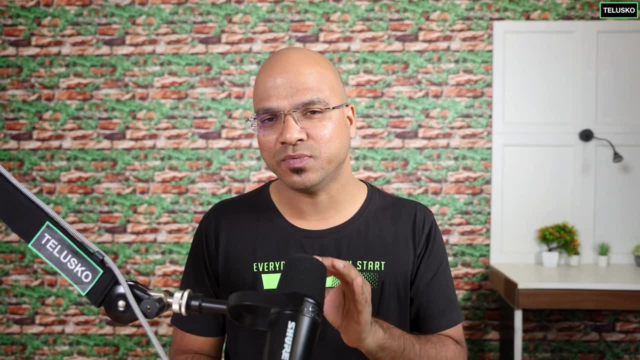 thinking, uh, my computer is super fast, it will be happening very fast there. see, in the world we have different computers and different computer have different cpu power, different ram power, different configuration, and that's why let's not calculate the speed of our speed, of a code or the 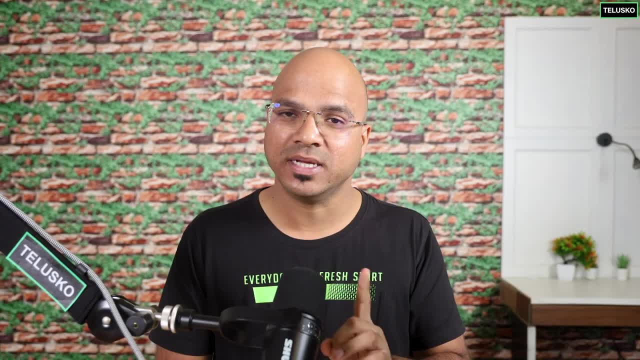 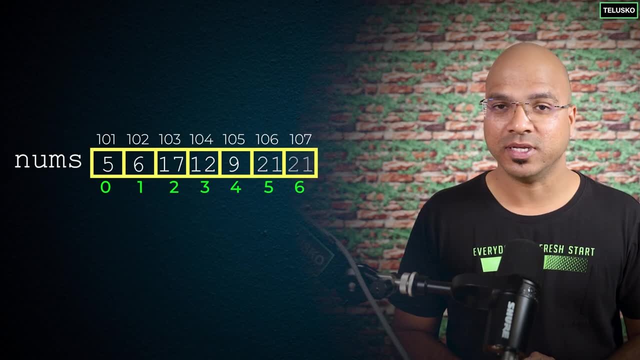 algorithm by the actual runtime. important is the number of steps it takes. example: let's say: if you want to insert the element at the end, that's good. if you want to insert the element in between, that will take a lot of steps. it's because you want to move the elements, right. 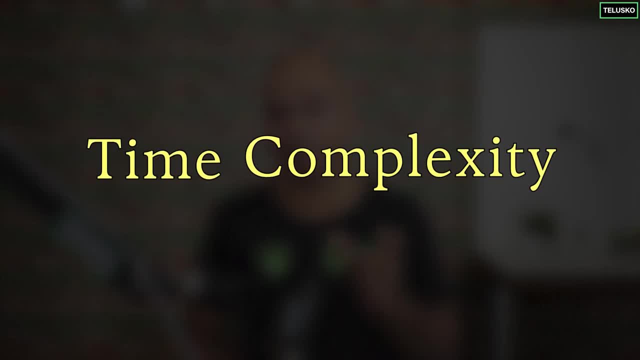 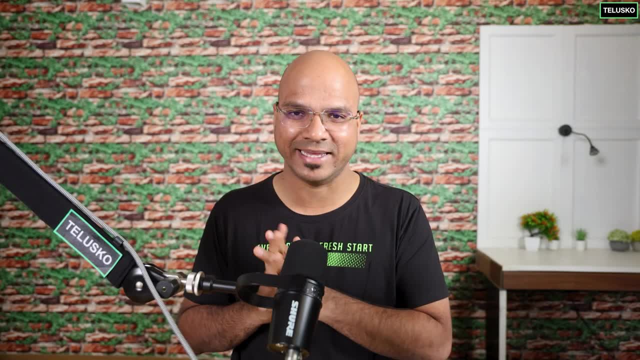 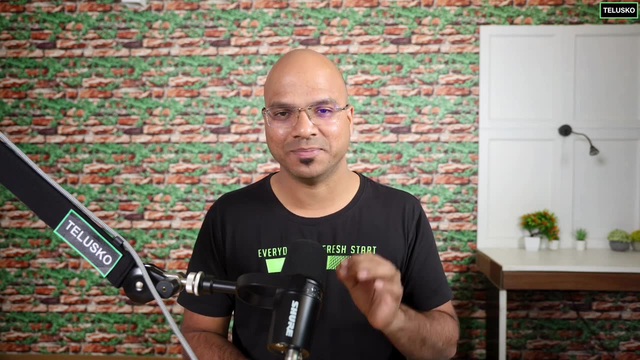 something called big big o notation. but yeah, we'll talk about that in detail later. i know you're excited to hear that. but important thing is, when you write a code, think about the number of steps your code takes, because that defines your time, complexity and if you say, my algorithm is good. 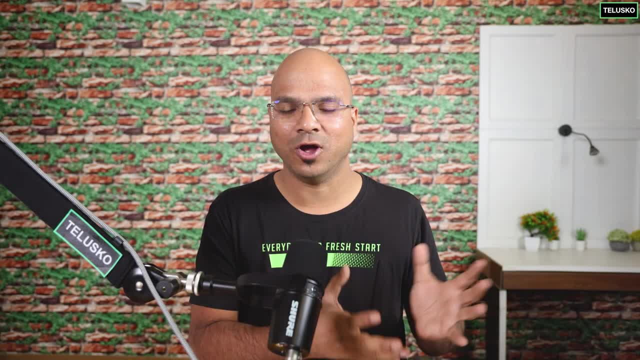 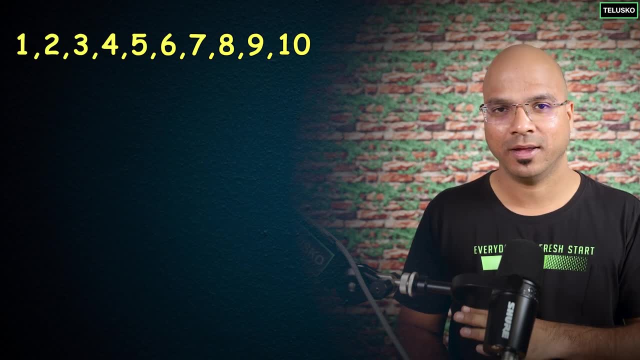 it should be time efficient. okay, so for the same particular operation you can write two different codes. example on the screen: if you want to print, let's say, 10 numbers from 1 to 10, and maybe you just want to print the even numbers, we have two options there. 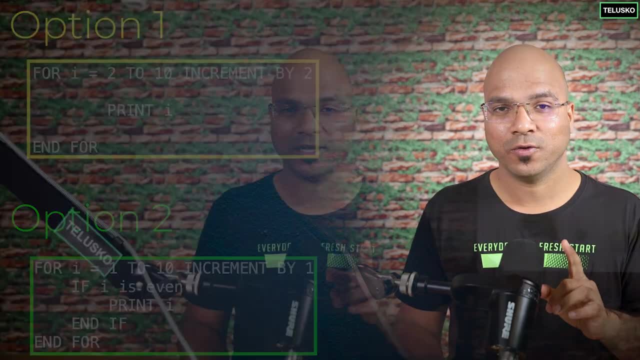 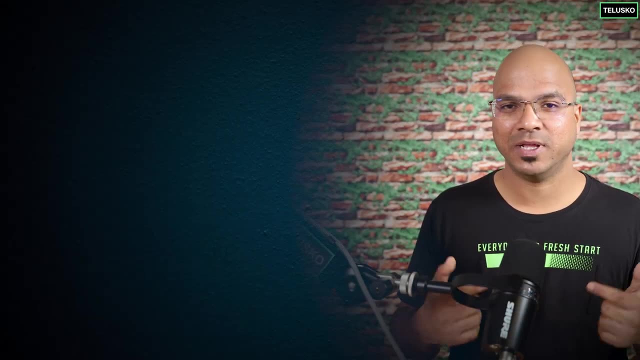 which one is good, of course, you let me know in the comment sections. but the code which is not trading between all the values is good, right. so that's how you define how your algorithm is good. now we can also expand the example. let's say: if you have a sorted array, so let's say you have an. 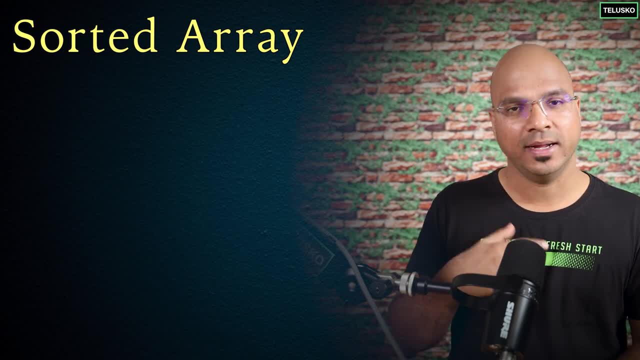 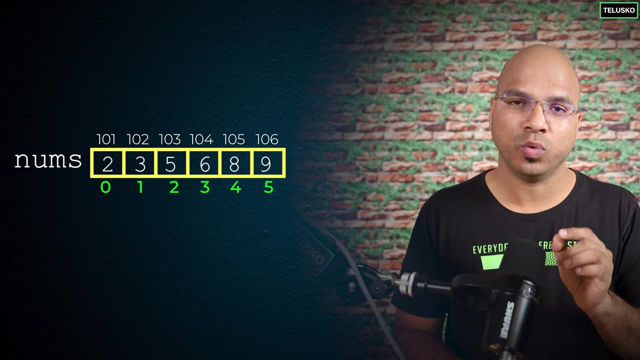 array and this is sorted by default. so every time you insert the element, it gets sorted by by default. you don't have to mention where you want to insert this example. let's say you have a bunch of values here, all are sorted, and now you want to insert the element which is 11. now, if you want to insert 11, 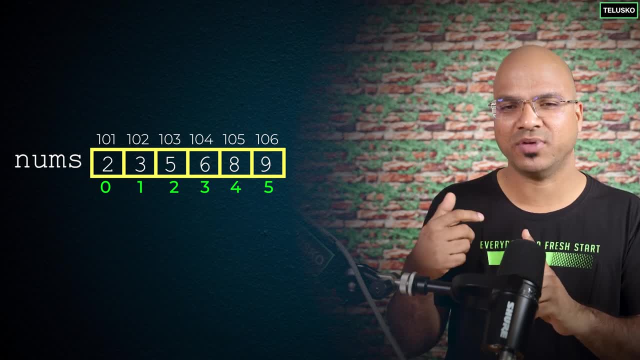 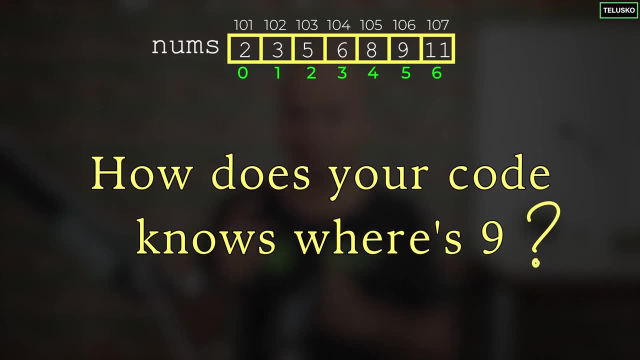 there where it will get inserted. of course it will search for the location. let's say we have a number, 9. it will get inserted after 9. now the question is, how do your code knows where is 9? so you have to basically search, you have to match: is it greater than? is it greater than? is it greater than? and then 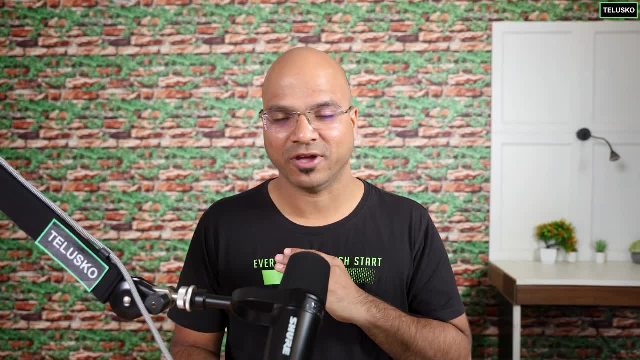 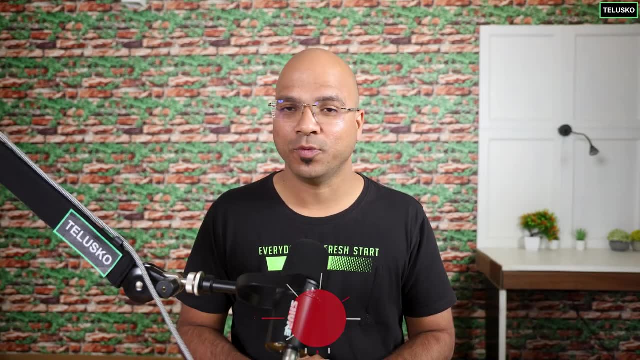 you have to insert, so that will take a lot of time. but what if you're inserting in between? you have to shift all the elements. so that's about the array and a basic introduction of time complexity. we'll discuss that in detail later. so i hope you enjoyed the video and in the upcoming videos we'll talk about more about. different data structures. 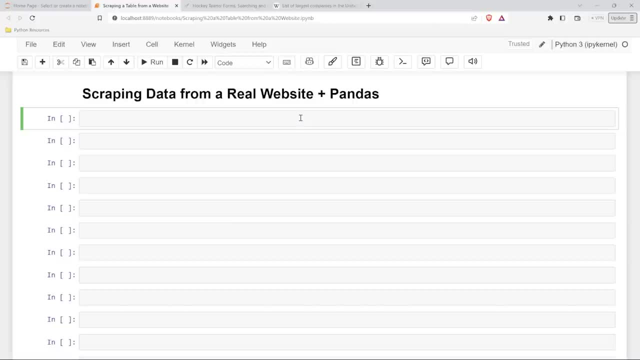 Hello everybody, In this lesson we are going to be scraping data from a real website and putting it into a pandas data frame and maybe even exporting it to CSV, if we're feeling a bit spicy Now. in the last several lessons we've been looking at this page right here And I even 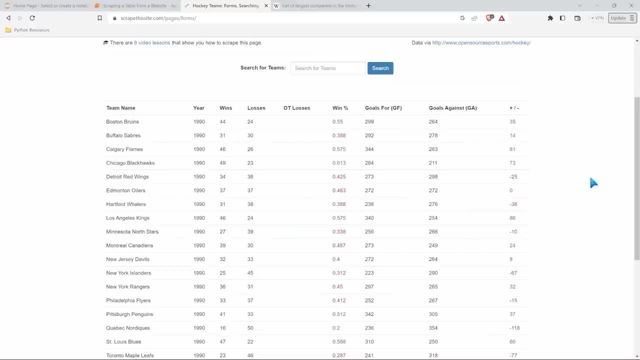 promised that we were going to be pulling this data, But as I was building out the project, I just I honestly thought it was a little bit too easy, since in the last lesson we kind of already pulled out some information from this table, And I want to kind of throw. 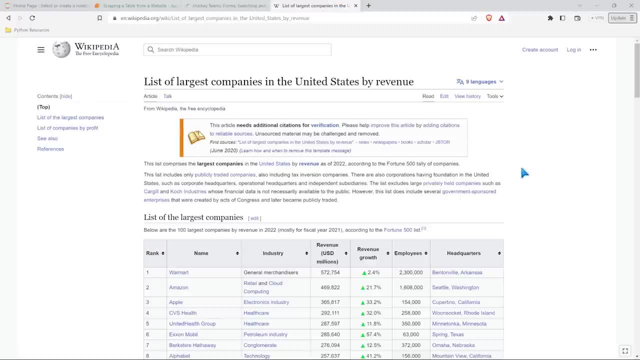 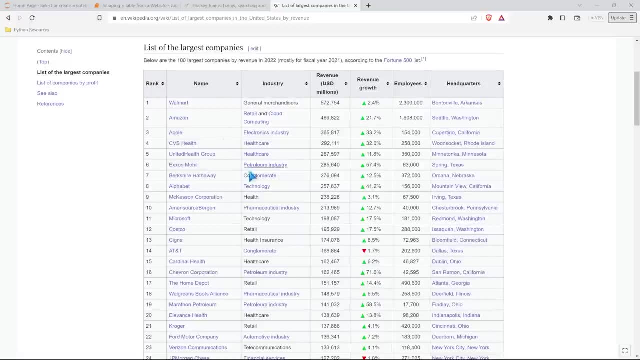 you guys off. So we're going to be pulling from a different table, We're going to be going on to Wikipedia and looking at the list of the largest companies in the United States by revenue And we're going to be pulling all of this information. So if you thought this was going to be easy and a 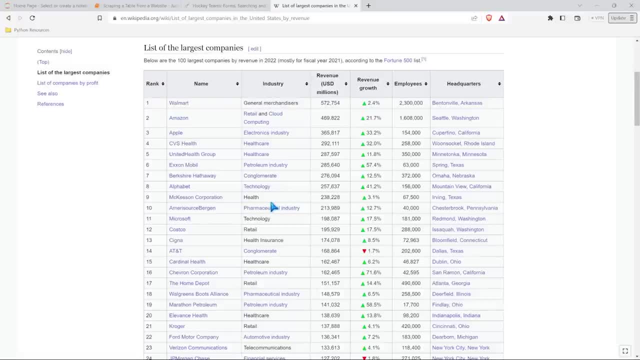 little mini project. it's now a full project, because why not? So let's get started. What we're going to do is we're going to import beautiful soup and requests. We're going to get this information and we're going to see how we can do this, And it's going to get a little bit.